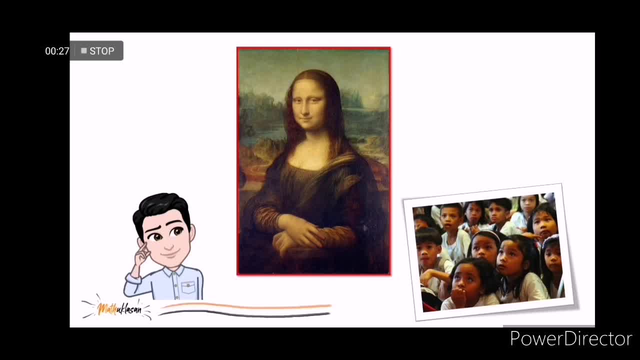 a mathematician uses numbers, patterns and equations to express the beauty of nature. And we don't have to be that good to see the world using mathematics. We ourselves can demystify the universe if we could just see patterns in nature. 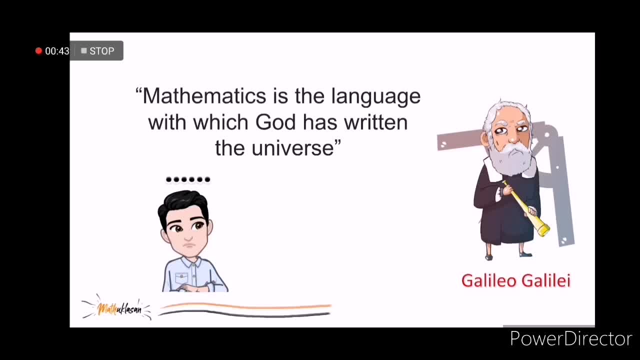 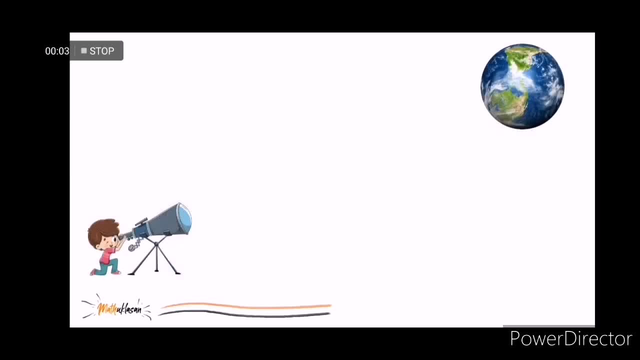 Well, even the famous astronomer once said: mathematics is the language with which God has written the universe. If you want to understand the world using math, there are three steps to follow. First, you need to find patterns, Then you need to. 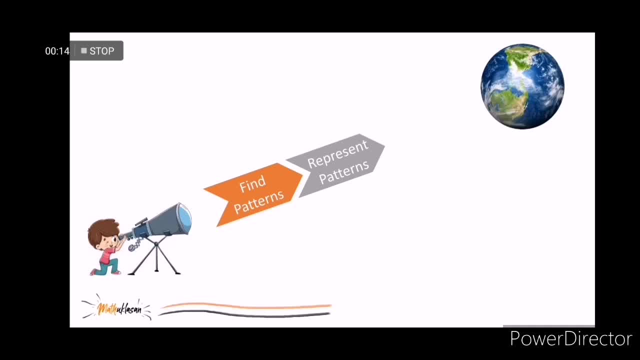 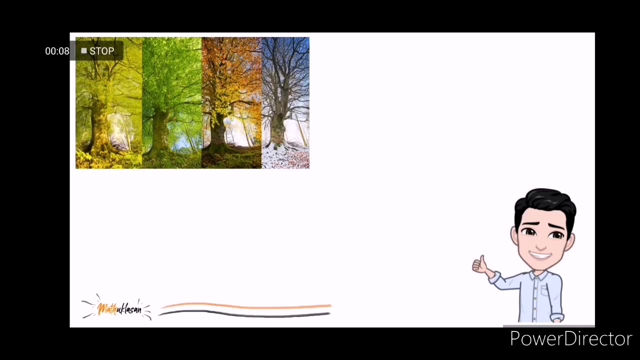 represent these patterns in the form of symbols, notations, shapes or numbers, And finally interpret these patterns. There are many patterns around us. In countries with four seasons, the sequence is always winter, spring, summer and fall. Our body follows a natural internal process that regulates the sleep-wake cycle and repeats 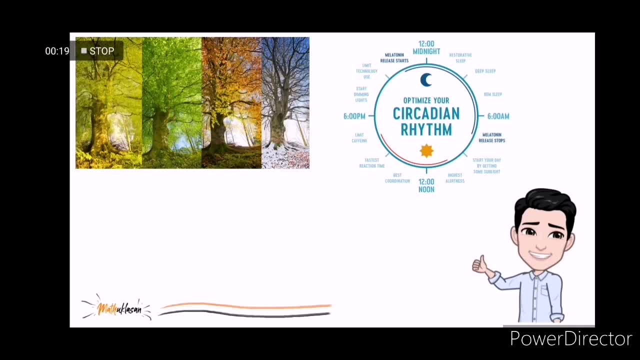 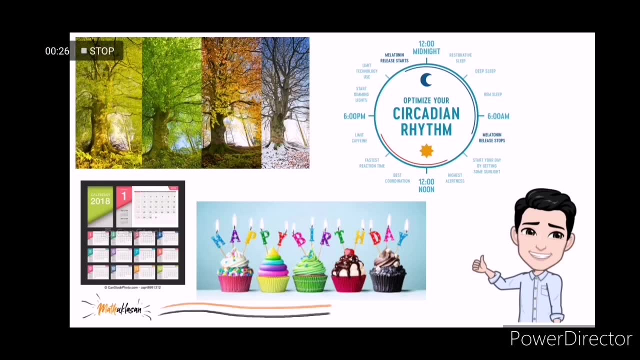 roughly every 24 hours, which is called circadian rhythm. And how do we know when to celebrate our birthday? By looking at the calendar. They have been in use for over 2,000 years. This suggests that thousands of years ago, people had already discovered patterns of time and 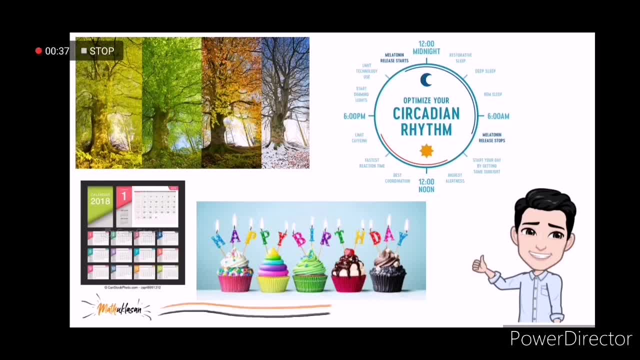 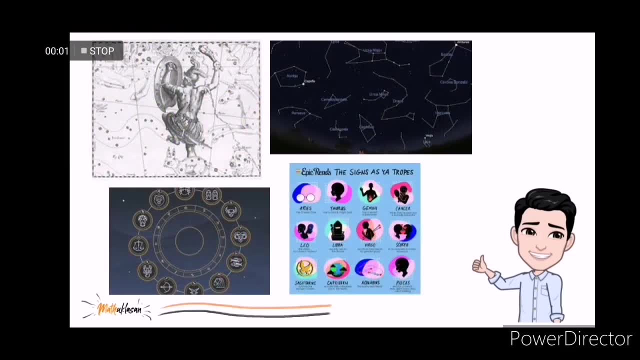 seasons It affected when they planted, harvested, hunted and performed many other tasks necessary for their survival. When you look up the sky, you may see different constellations. These patterns, for example, were devised by poets, farmers and astronomers to identify stars and their locations. 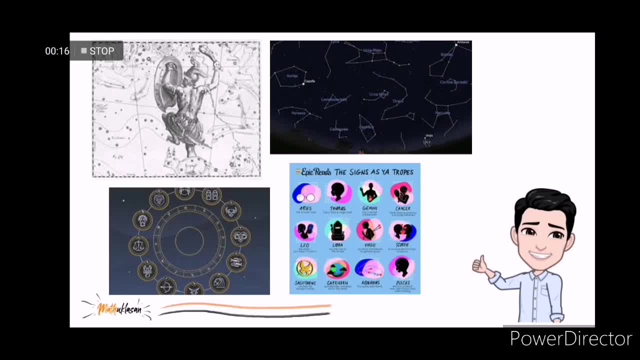 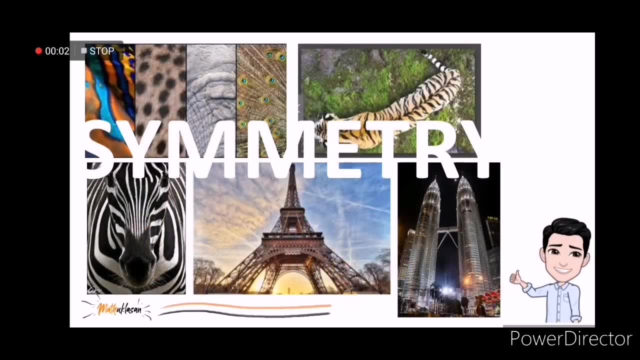 On the other hand, the 12 zodiacal constellations, or the signs of the zodiac, are famous today for their use in astrology. It is also interesting to know that these patterns of nature are being used by humans in designing magnificent structures. 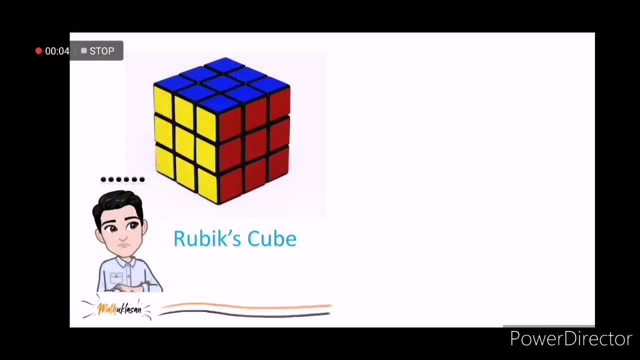 Have you ever tried solving a Rubik's cube? It may seem impossible to solve it at first, but there are various patterns that can be used to match all the colors. These rotation patterns that are available in the internet are coded as seen on the right side. 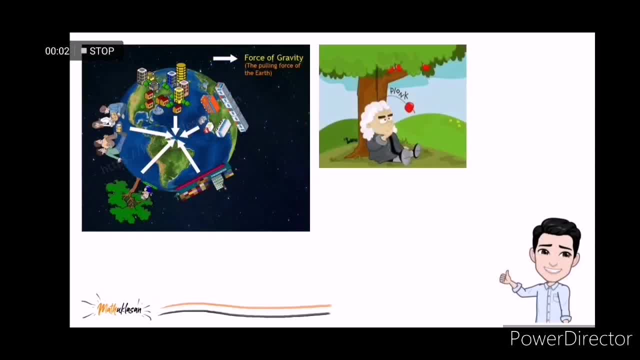 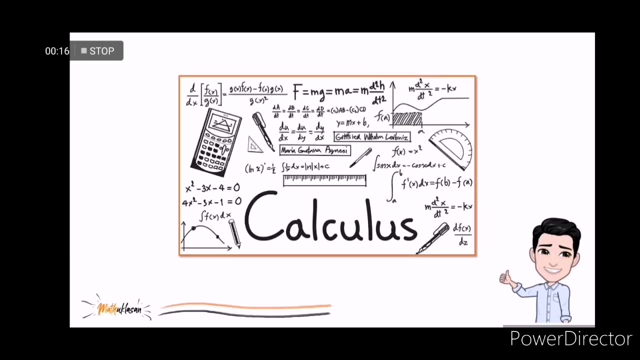 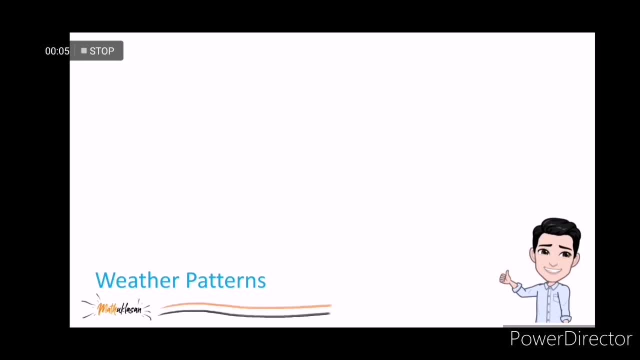 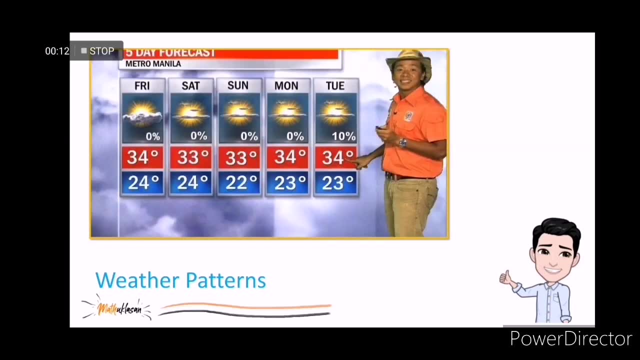 5. The Future of Mathematics. 5. The Future of Mathematics. The future is something that we can't predict, But how can the weather forecasters tell the possible weather conditions of the coming weeks? That's because of weather patterns. They were derived from the previous data that they had. 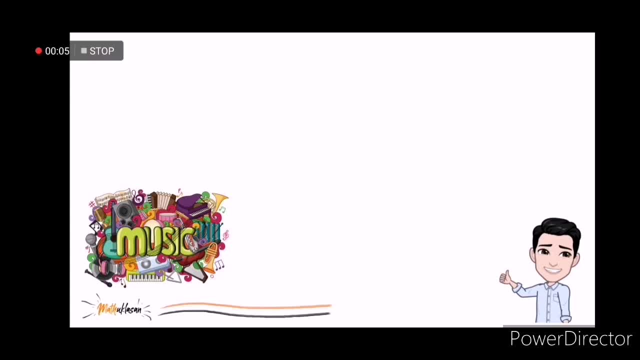 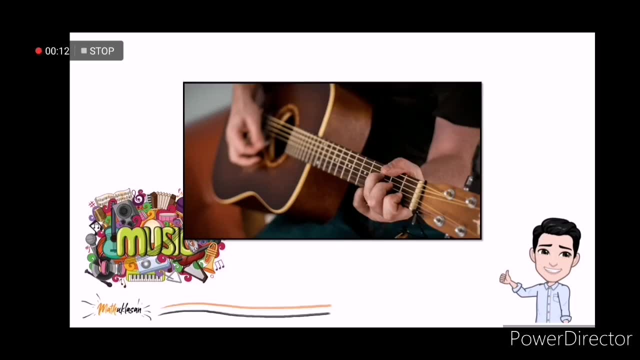 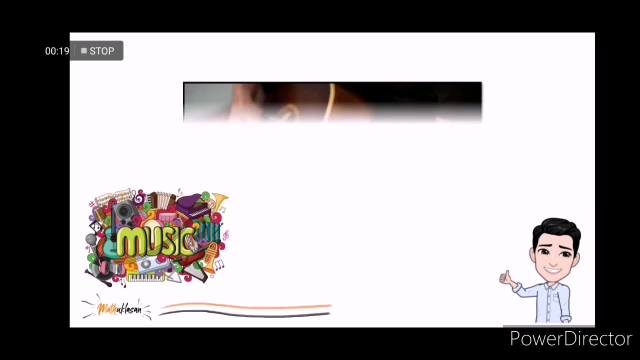 And who doesn't love music? Many considers music as a form of art, but technically it is a collection of coordinated sounds. And what better way to produce these sounds? Musical instruments like guitar and piano. Compositions in guitars are visualized using tablatures in which notes and numbers are used to show the 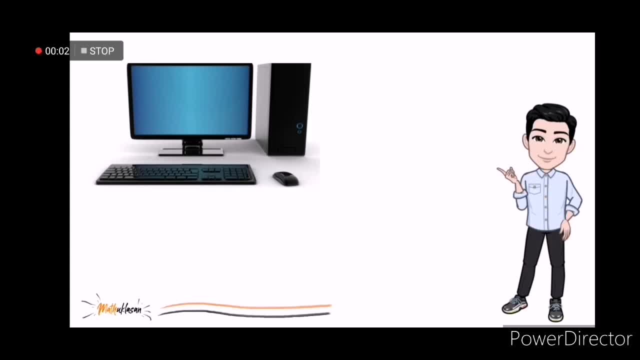 progression of sounds. Do you know that when you type a word on your keyboard, the CPU reads it differently? The language of a computer is represented by zeros and ones called binary digits, So a computer uses thousands of binary patterns to process any inputs. 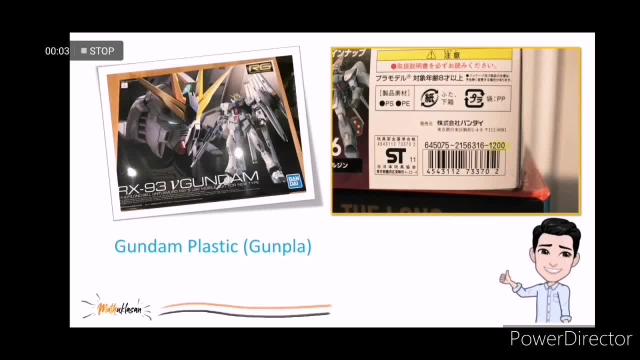 6. The Future of Mathematics. 7. The Future of Mathematics. I'm a Gunpla Builder and in the previous years the Mathematical Institute of the University of Physics announced a method with which the computer needs to interpret. слово- puerto TEK. 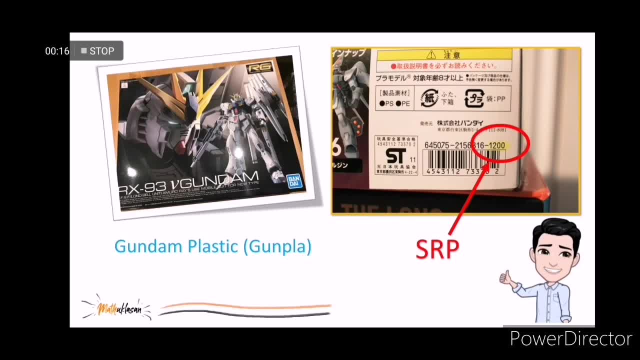 but cannot measure tremSpe because it requires any meals or none. How is the feather supposed toıs? Just add any possible formula or Carol, like the Accent, A chord or an verb, and square знач goes to S. with that formula you can вход Sense in encalpment in. the numpm parameters. It means the cell into the cell size. is thegrba I where diet goes and up goes the spread grade? is it in H, such as Q4.. Just type and explain: sparks and winds effect P, Pp or G. 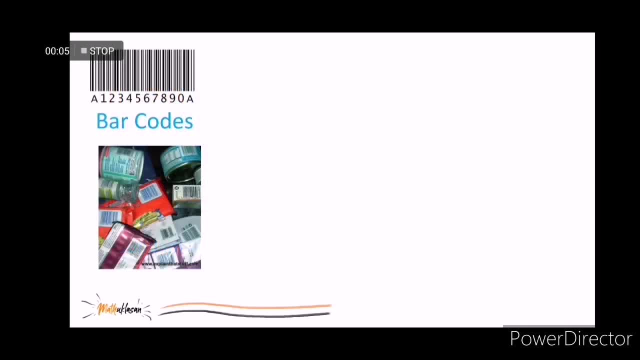 Barcode is a readable optical label that contains information about the item to which it is attached. This is what the cashier in the grocery uses to include each item in the transactions. A 2-dimensional barcode issues will for that BARCODE, which includes: which is a test of quantity. 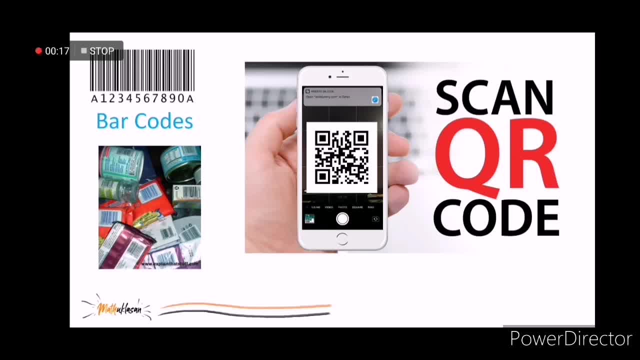 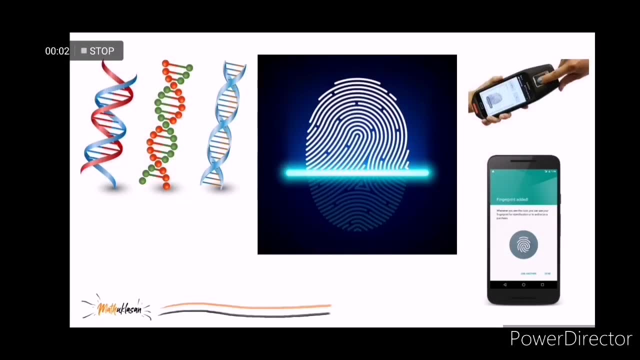 barcode, called QR code, consists of black squares arranged in a square grid on a white background, which can be read by an imaging device such as smartphone camera. today, QR codes have become common in consumer advertising. there are also many unique patterns in our body, like DNA and fingerprints. no two people have exactly. 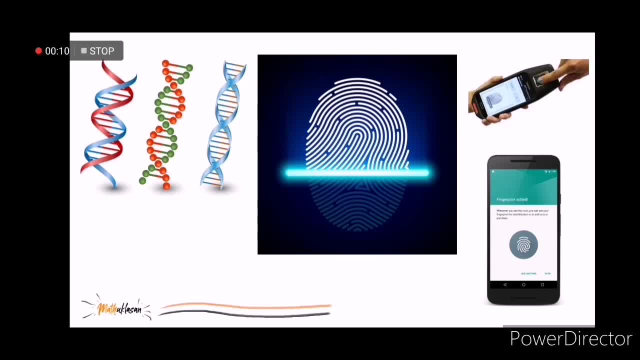 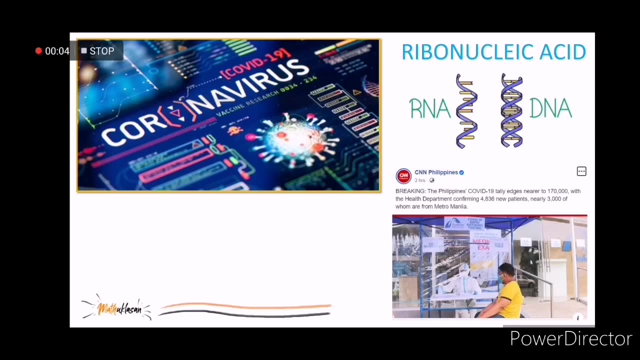 the same fingerprints. fingerprint analysis has been used to identify suspects and solve crimes for more than 100 years. now it is also used for biometric security systems like the one in your phone. coronaviruses are named for the crown, like spikes on their surfaces. coronaviruses have all their genetic materials in something called RNA- RNA. 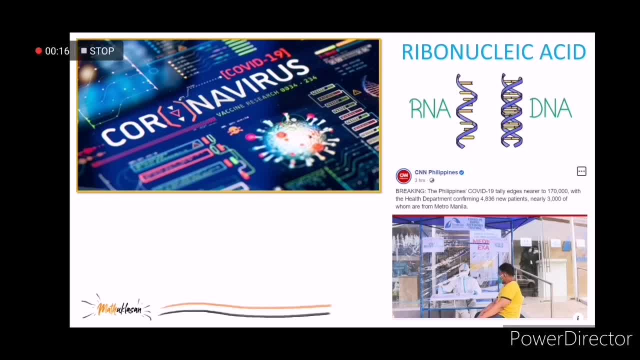 has some similarities to DNA, but they aren't the same. the constant changes in their RNA patterns result to the other strains like CDA, SMR, AVG, buteten, ferrum, hemoglobin of the respiratory system, receptors and effects of asbestos and other neurotypersial genes. 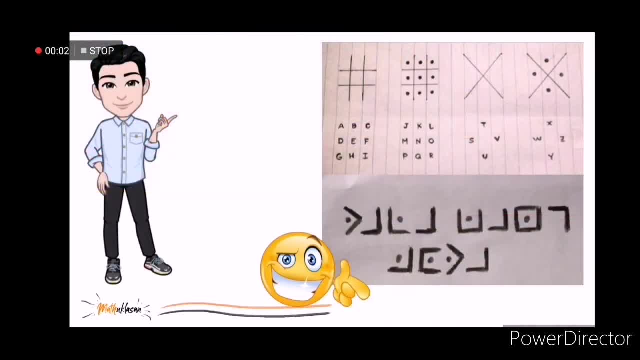 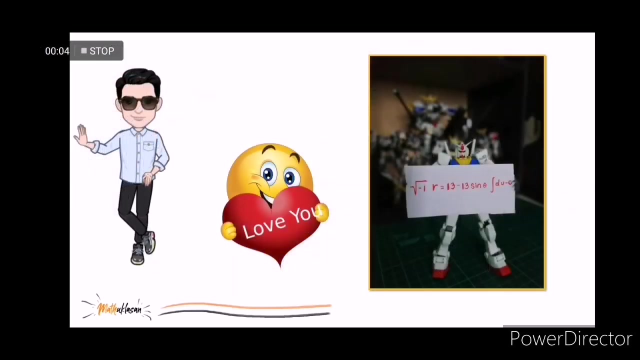 the COVID-19. and do you know? other people create their own patterns, for fun or for communicating secretly. i found this one on facebook. you can pause the video if you like, but if you want a hint, well, it's a status and in my case, i use my knowledge in math to express secret messages. 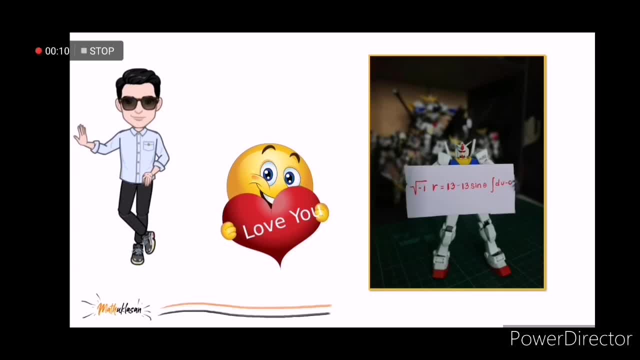 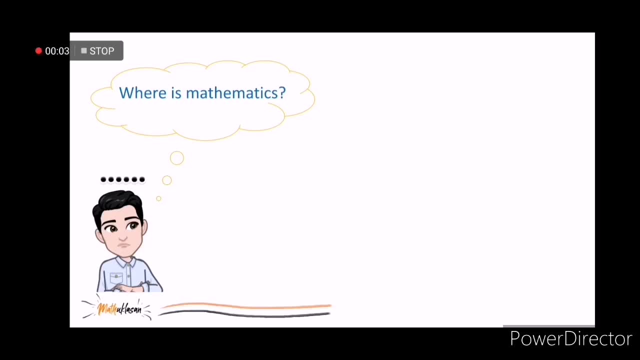 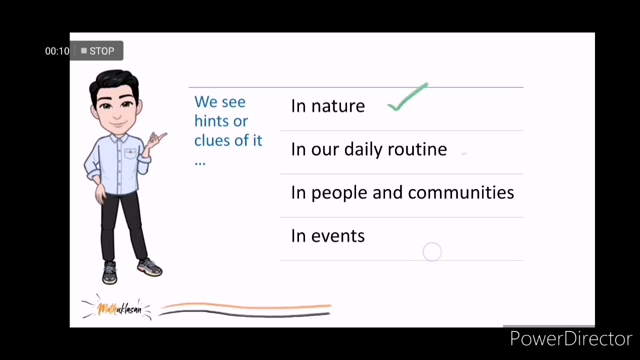 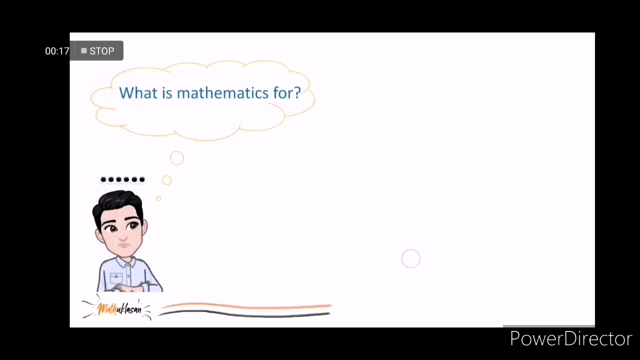 to my loved ones. well, not so secret if you know math, cool stuff, huh. so, with all these things in mind, where is mathematics from a right viewpoint? mathematics is in nature, in our daily routine, in people and communities, even in events. what is mathematics for? math helps us unravel the puzzles of nature. 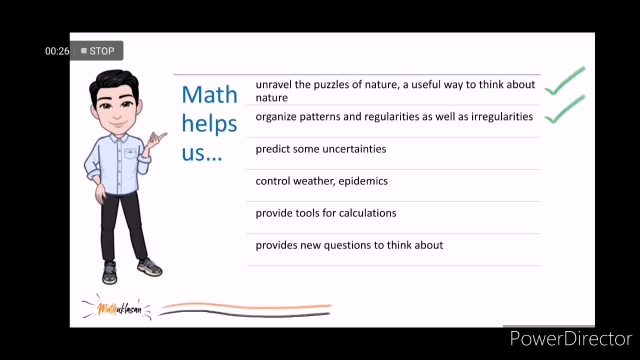 or math helps us solve the puzzles of nature, or math helps us solve the puzzles of nature, or math helps us unravel the puzzles of nature, or organize patterns and regularities, as well as irregularities, predict some uncertainties, control weather epidemics, provide tools for calculations, provide new questions to think about. 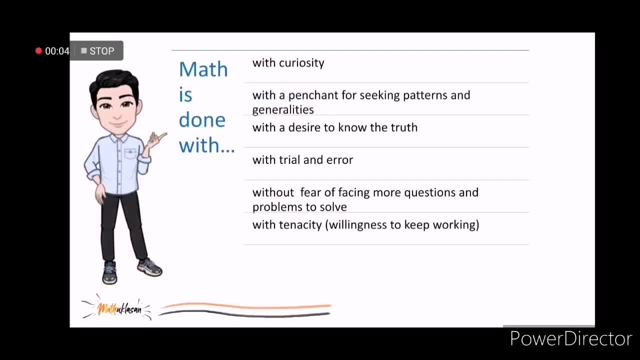 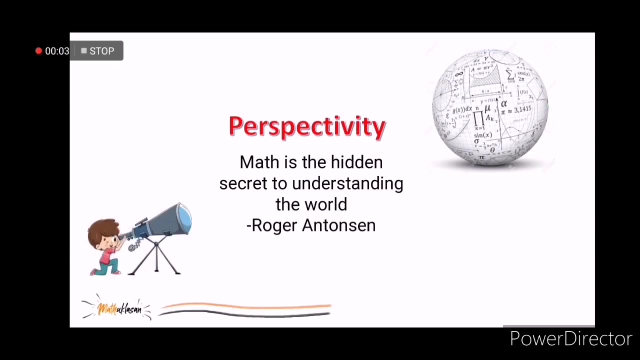 now, how is mathematics done? math is done with curiosity, with a penchant for seeking patterns and generalities, with a desire to know the truth, with trial and error, without fear of facing more questions and problems to solve with tenacity. so why not try to see math from a different viewpoint, and maybe 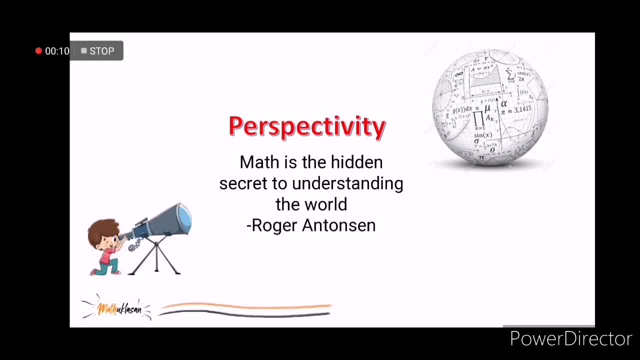 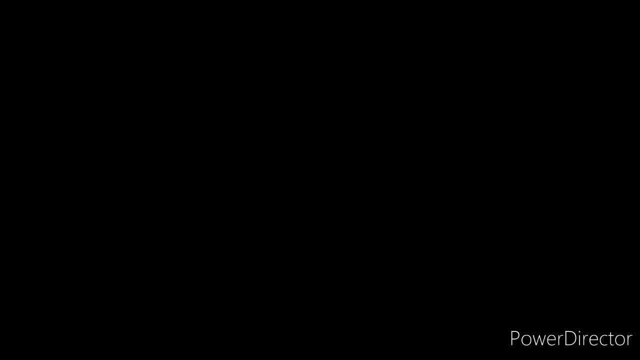 it is the hidden secret to understanding the world, and let us discover it together. thank you for watching you.